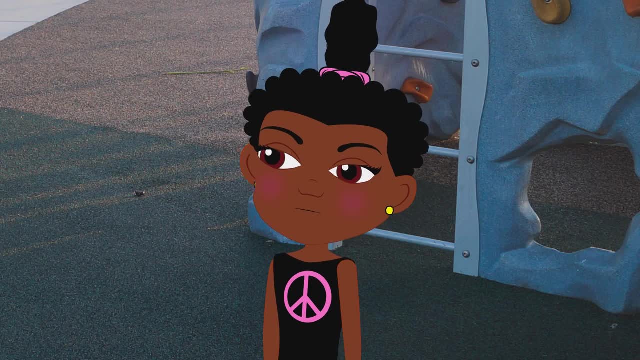 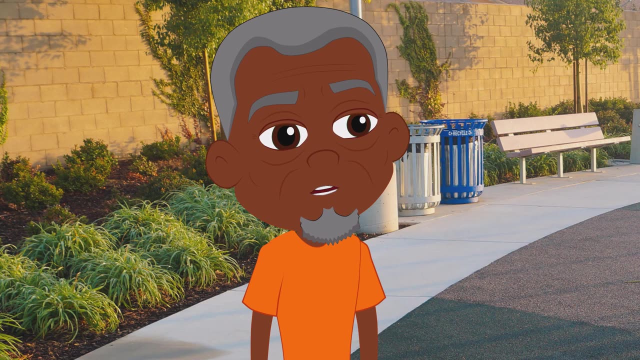 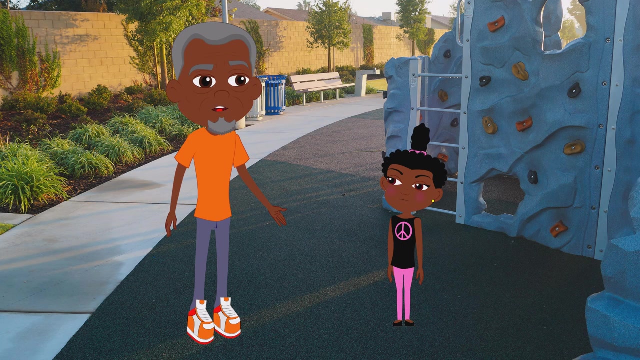 that everybody goes crazy for A new car, a new house, new clothes or even how you kids go crazy over them cell phones. That's just people. But if you work hard for your money, you want to make sure you spend it wisely and even save some, I guess. All right, then, don't waste your money on. 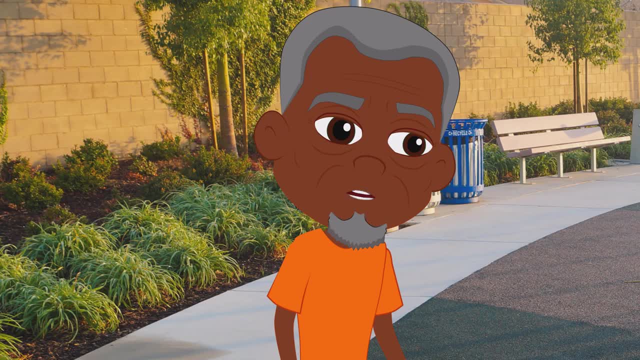 the latest fads, especially on something you don't really like. Save your money, it's important, But, Mr Rose, don't we work just to save money, Mr Rose, don't we work just to save money, Mr Rose? 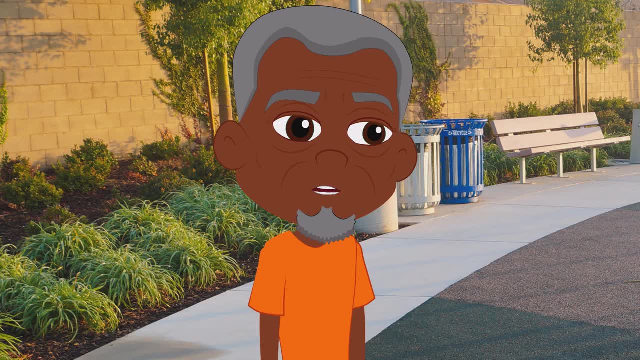 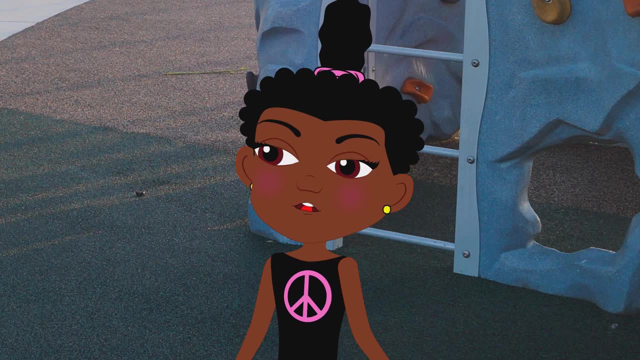 don't we work just to have it to spend? Yes, little lady, Many people work hard to get money to buy things. but if anybody knows, I know there is nothing worse than being broke. I know right. My mom is always so sad when she has spent all of her money and can't take us anywhere because 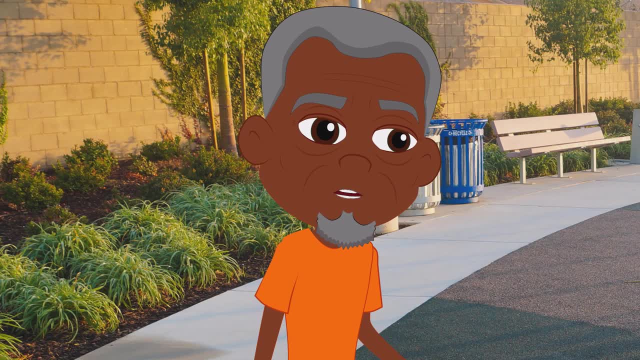 she's broke. I have been there. That's when I had to learn how to figure out when to save and when to spend. How do you know that, Mr Rose? Well, when I was a kid, like you, I would help my dad. 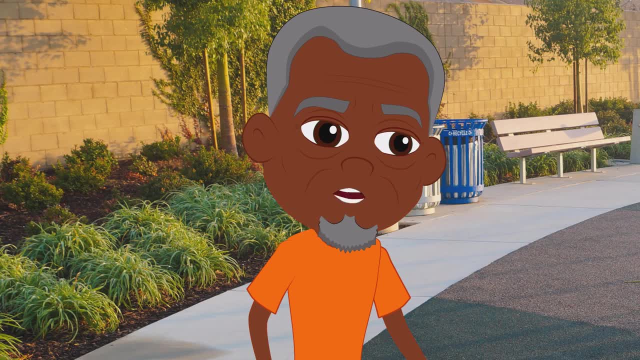 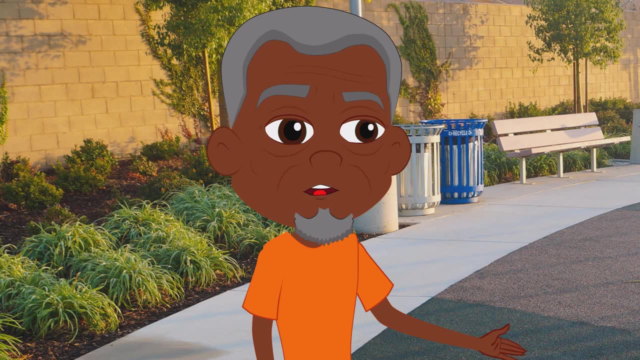 with mowing lawns. My dad taught me that every time he pays me some money, I have to save. Each month he gave me $10 for helping out. Out of that $10, I would donate $1 to charity and then take $2 and put it away in a jar that I hid under my bed and left it there. so I had $7. 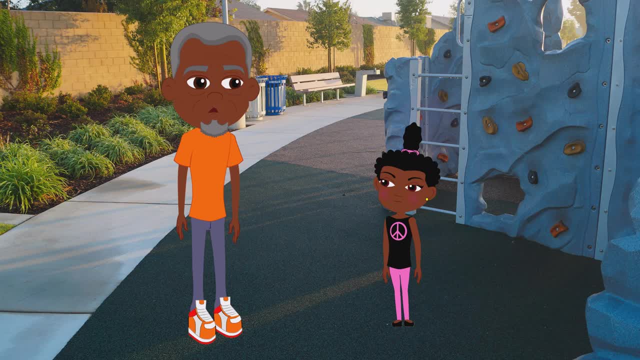 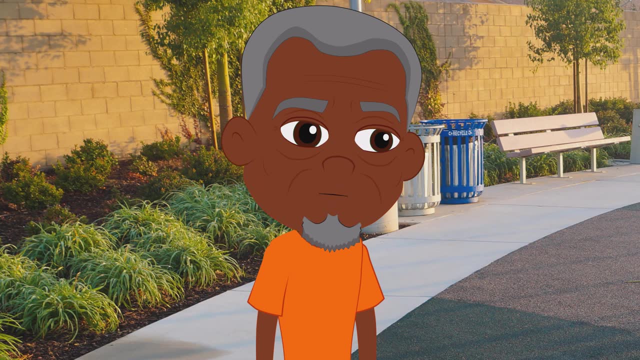 to spend when it was all done. Now, in five months, how much did I save? Well, if you save $2 for five months in a row, that is $10.. That's right. I'm not saying to not enjoy your money, but don't blow. 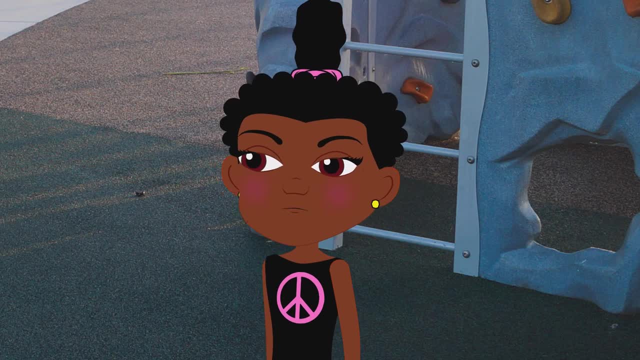 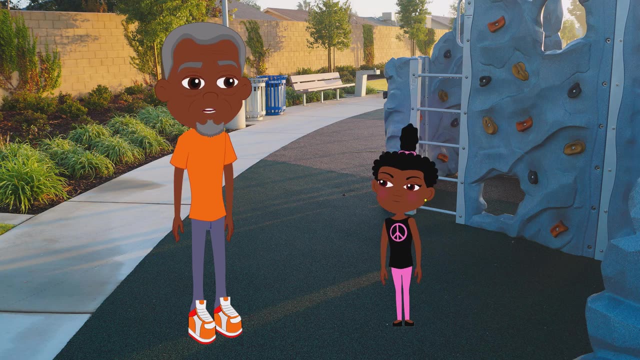 it all on simple things. when you can save for a rainy day, That makes sense. Mr Rose, I'm not saying that Great little lady. What I really want you to understand is: don't be so quick to spend your money, but be wise about what you buy. That money that we receive is a tool to help. 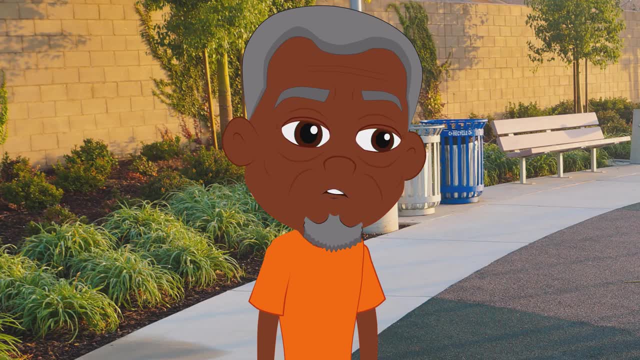 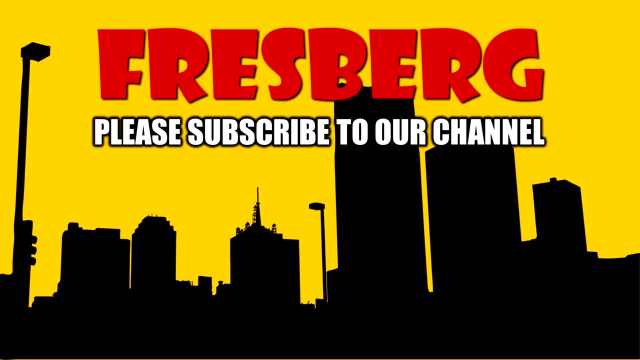 others. buy what we need and prepare for the future. Thank you.